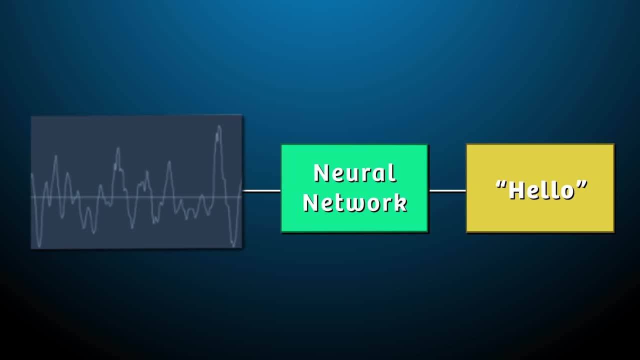 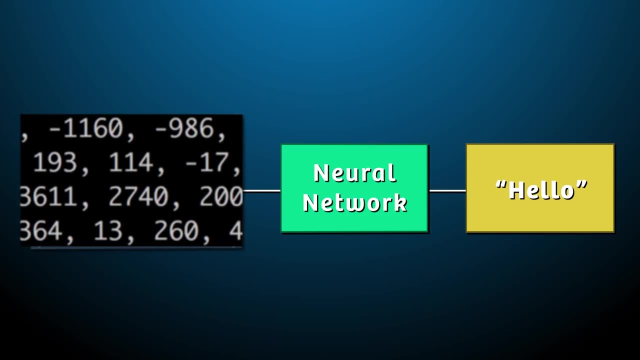 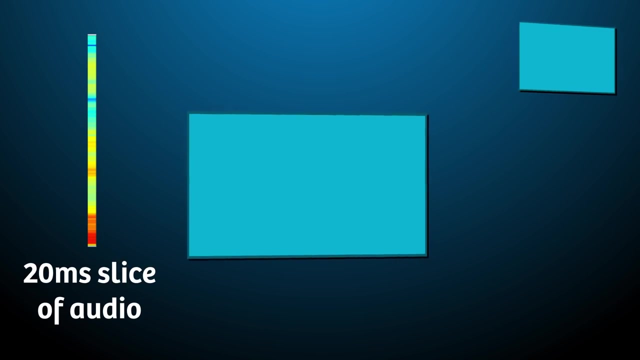 dataset of audio clips with their transcripts as the labels. Every single byte of the audio can be broken down into a series of numbers, and so can the text transcripts. One combination of operations will convert the input to the labels, and that combination is the function. 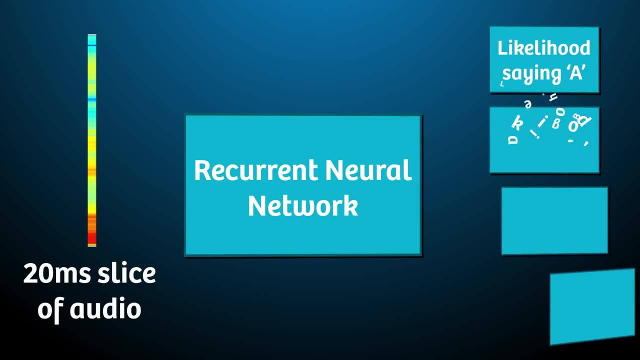 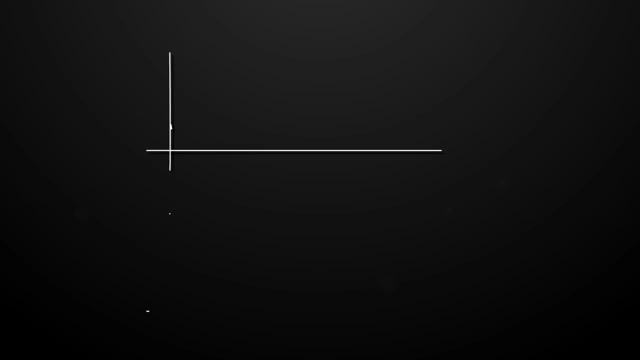 Neural networks can slowly approximate or get closer and closer to this function through an iterative optimization process, also called training. In short, it's minimizing an error value at every iteration so that, given a novel audio clip, it can easily predict what the transcript for it would be. 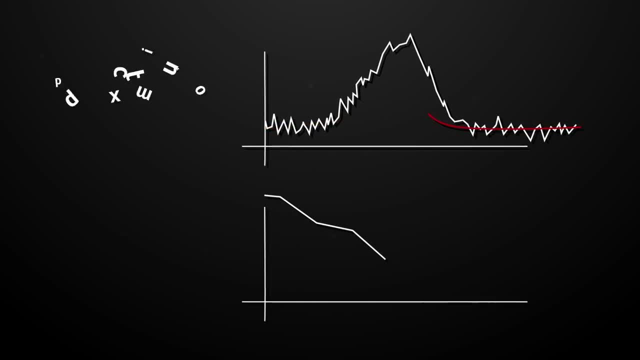 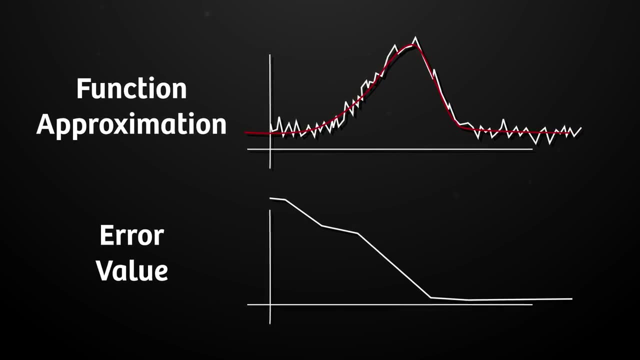 Deep learning is essentially performing A to B mappings. That's it. A more accurate way to say this is that it's performing universal function approximation, meaning with sufficient data, it can approximate any function: Input: a loan application. output: the likelihood a customer will repay it. 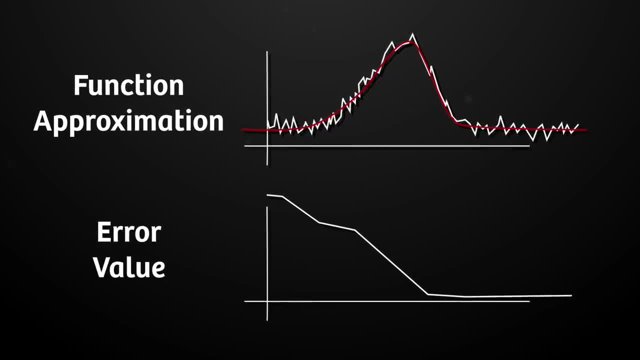 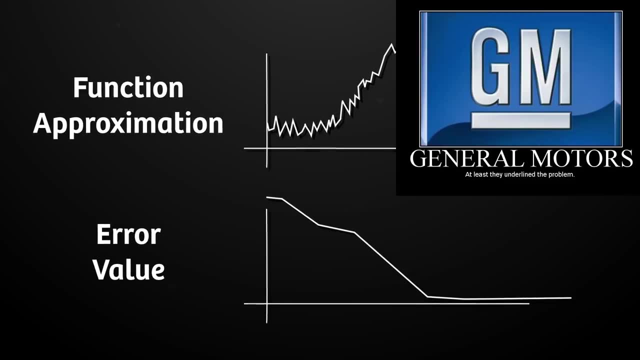 Input an email and output the possibility it's spam or not spam. Input usage patterns for a fleet of cars and output where to send a car next, like the dumpster, if it was made by GM, Since there are an endless array of applications for this. 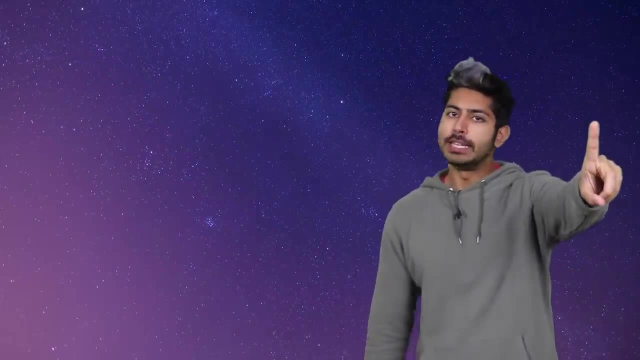 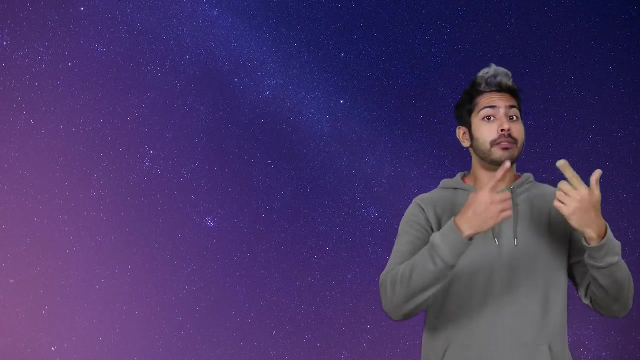 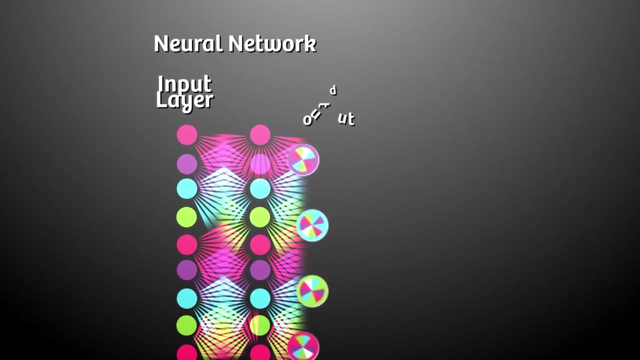 Deep learning has gotten really popular. But while deep learning is good at finding a function we don't already know, but have training data for, it's surprisingly useful to find a function we already know and then look at how we found it. All neural networks are composite functions. 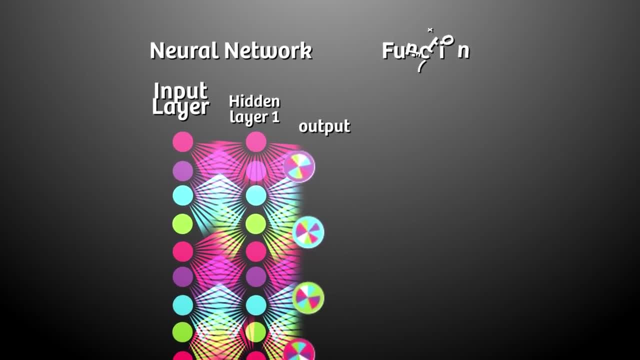 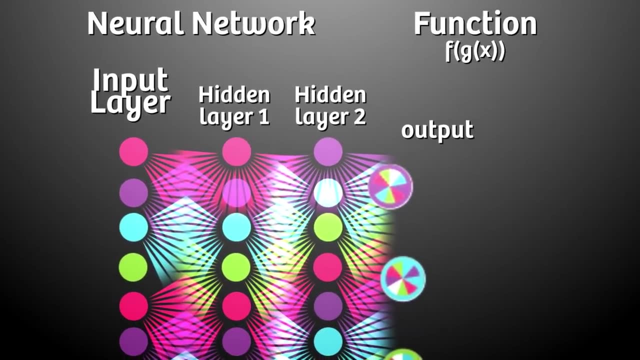 That means they are functions of functions. The more layers a network has, the more nested functions it has. For a three-layer network, we'd multiply the input by the first weight matrix, apply an activation function to it and repeat the process once again. 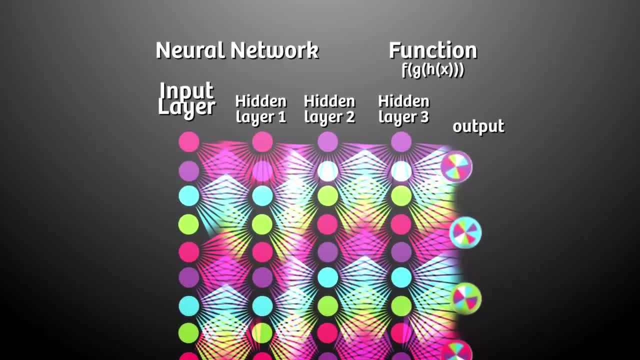 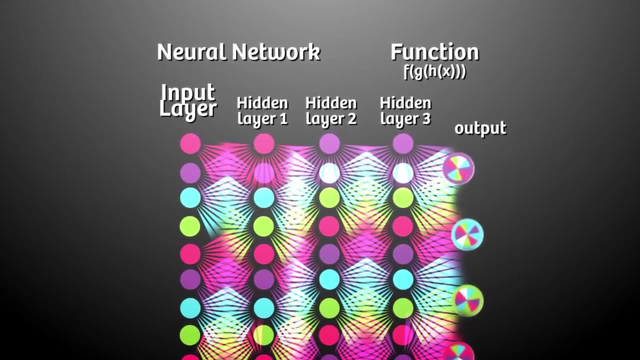 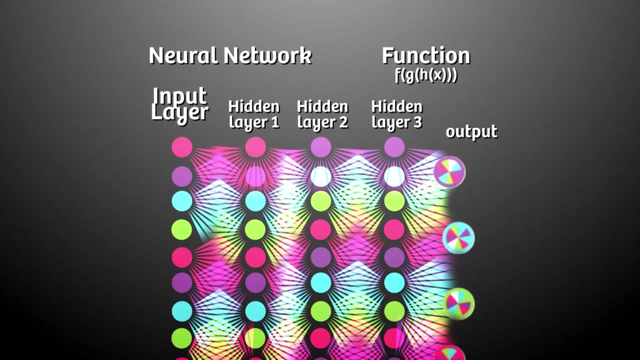 This time using the output as our new input Input times weight activate. The result is our output. This can be represented as a composite function, since we're using the output of the first function as input to the next function. But let's say our goal wasn't to find a label y, but instead to reconstruct the original. 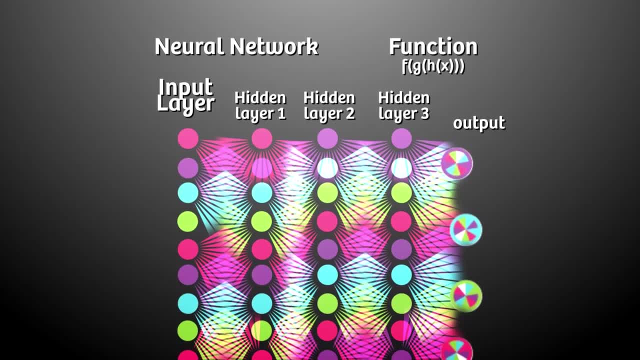 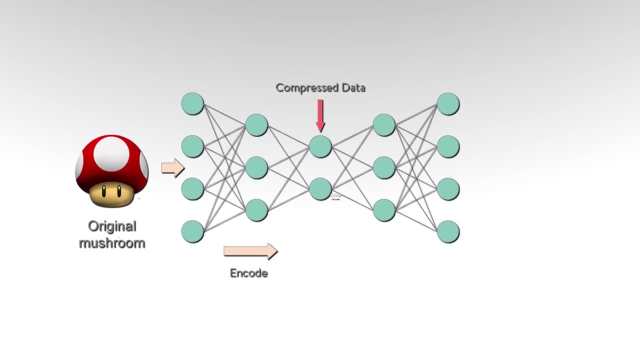 input x Meaning. if our input was an array consisting of a few numbers, our network should output that same input with those same exact numbers, after applying a series of operations to it. We can call the first part of the network that compresses the input into fewer bits. 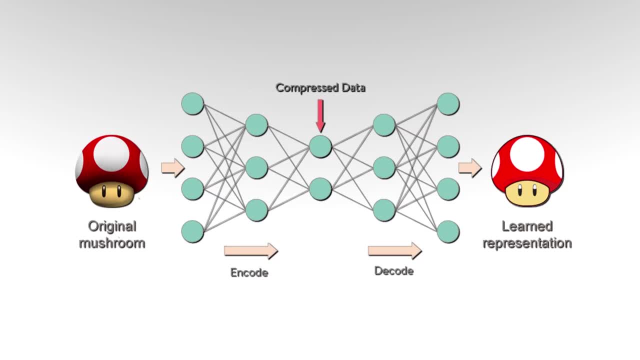 the encoder, and we can call the second part that reconstructs the image, the decoder. So why should we care about doing this? Well, we don't care about the output. it's just a replica of the input. What we care about is the hidden layer. 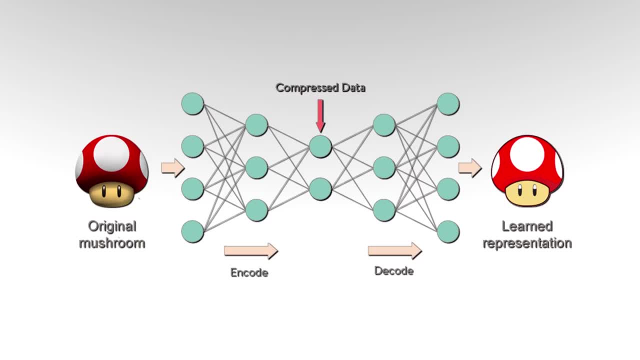 Once the network can reliably reconstruct its input, the hidden layer must contain a sufficient amount of information to represent the output. If, as is typical, the hidden layer is smaller than the input and output layers, what it represents is the same information in a lower density. 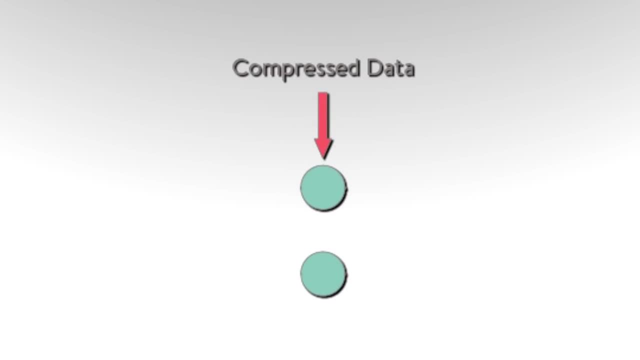 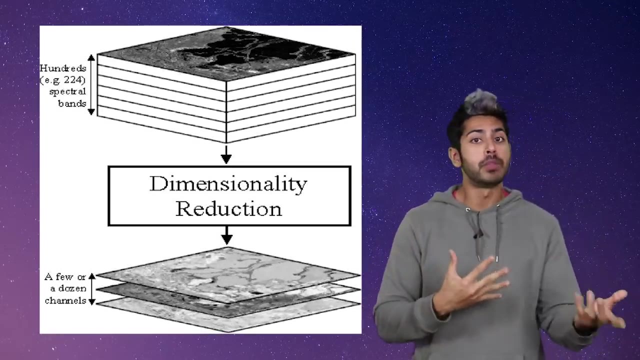 It's a much more dense representation of the input data, one that is learned over time. Although it turns out that there are better techniques for data compression, autoencoders are still really useful for some tasks, like dimensionality reduction. Subtitles by the Amaraorg community. 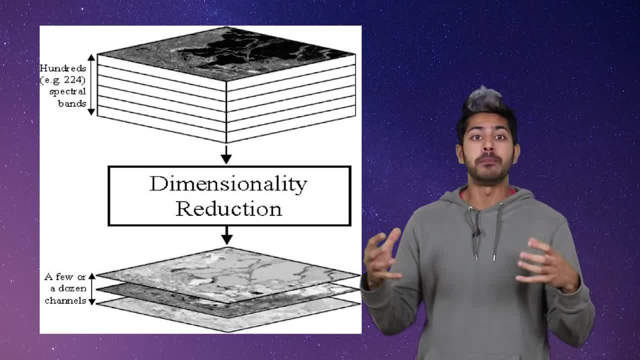 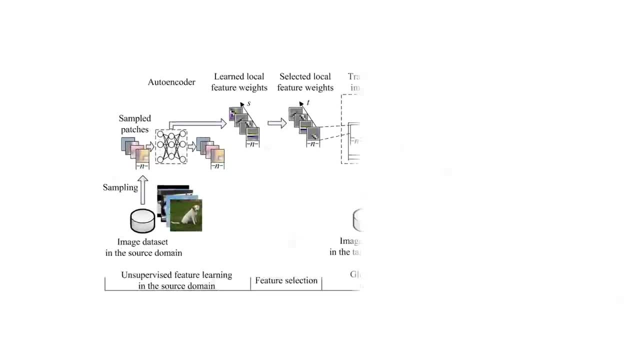 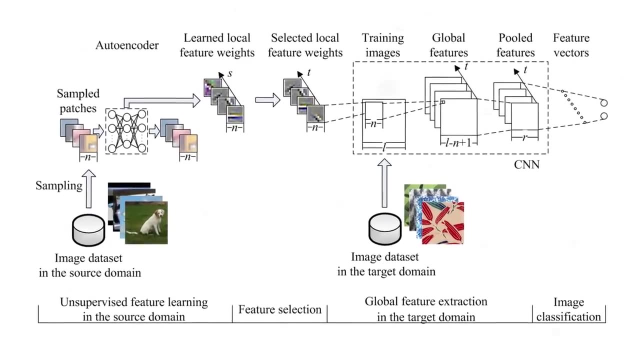 condensed representation of some multidimensional data. we can easily visualize it in just two or three dimensions for further analysis. We can also use it for classification. The idea is that we train an autoencoder to reconstruct its instances of a particular class. We don't train it on any instances of any other class. 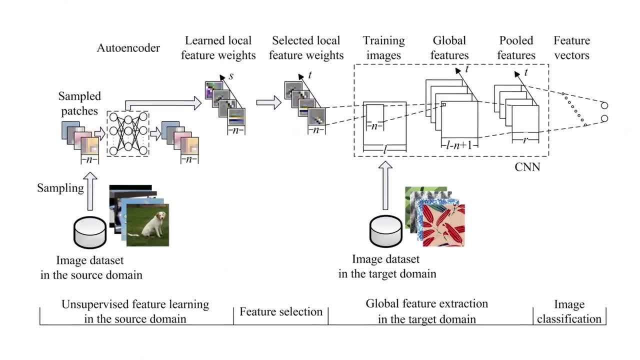 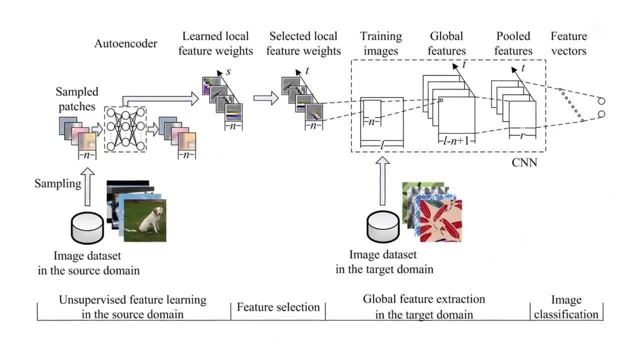 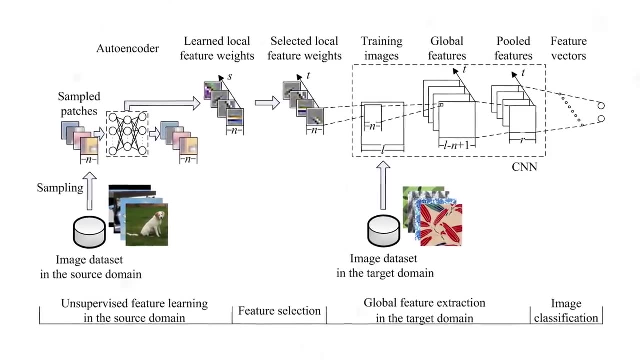 Then to classify new instances. we feed them to the autoencoder at the input layer, get a reconstruction in the output layer and compute the reconstruction error, which is usually a measure of distance between the reconstruction and the input. If it generalizes to a new instance and reconstructs it properly, then it's likely to be of the 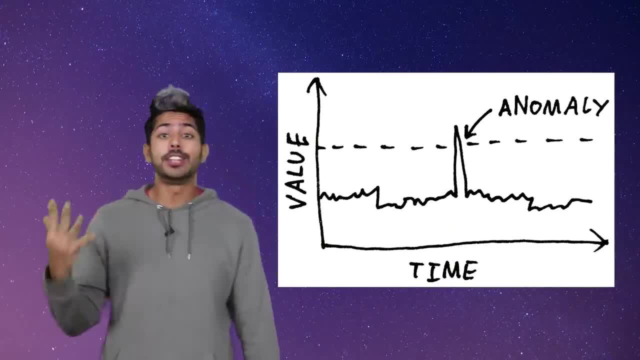 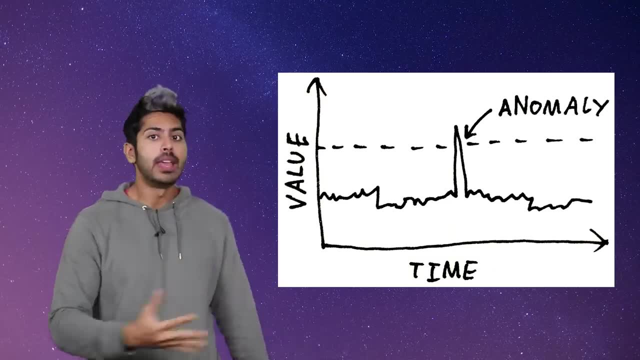 same class as the instance it used to train on. Anomaly detection is another use case. We first train it on normal instances so that if we feed it any anomalies they'll be detected easily. If we train it to recognize anomaly instances in our training set, it would only find the 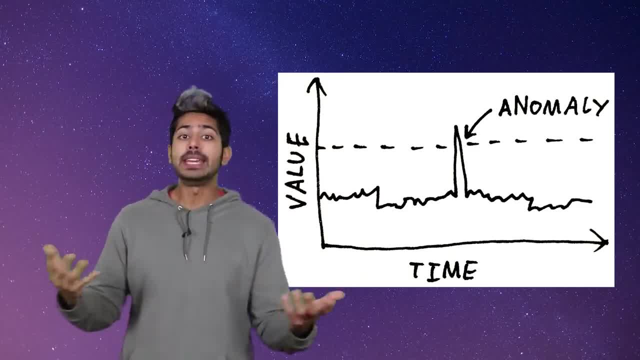 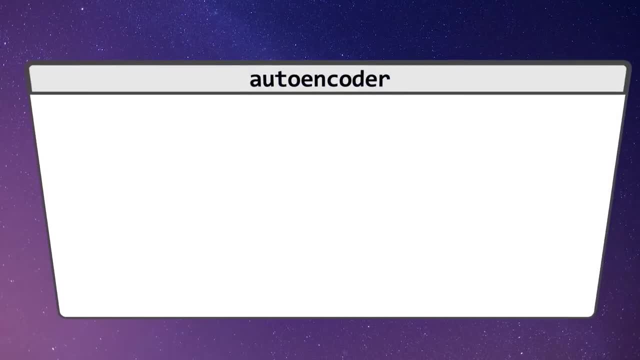 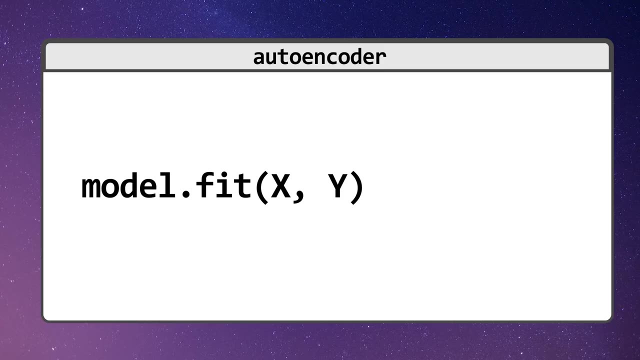 ones that look like anomalies. In many cases we have very few anomalies in our training set, but when using an autoencoder this isn't a problem. So autoencoders are just neural networks. where the target output is the input, We don't actually need any new code. 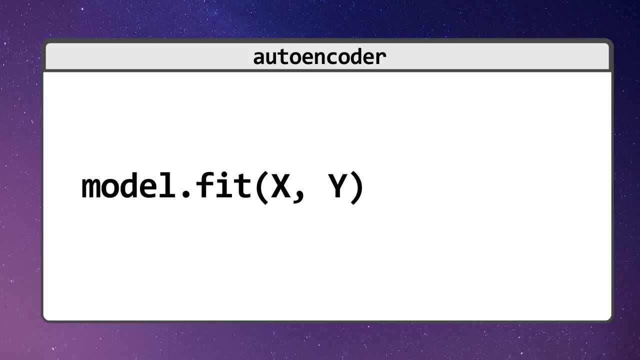 If we're just using a super simple scikit-learn-like interface, we'd simply train our model by changing a single parameter. Instead of modelbit x and y, we'd just say modelbit x and x. All the usual training strategies work with autoencoders. 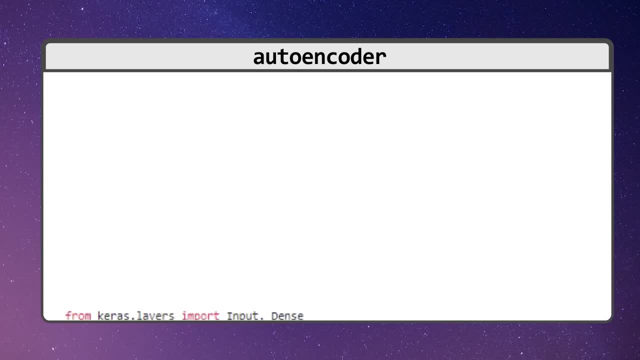 We don't need any new code. We don't need any new code. We use only the code we're given. It's not a problem to change the model. So what you can do is take that control over to your automation and build a new model. 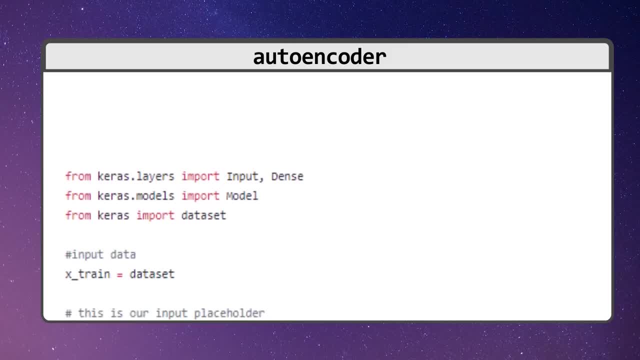 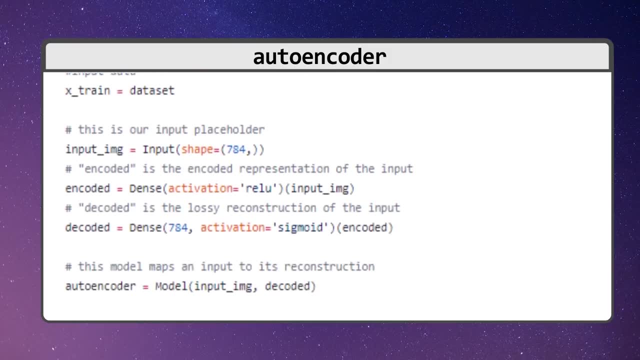 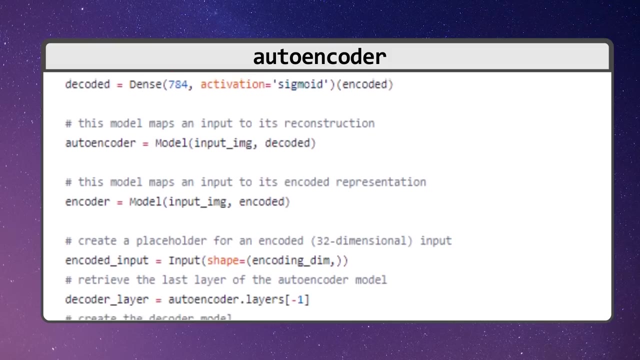 It's fun to take an existing neural network library and see what kind of low dimensional representations we can come up with If we were to build a really simple autoencoder using the keras deep learning library to reconstruct a training set of images. notice how a single, fully connected neural layer acts as the encoder. 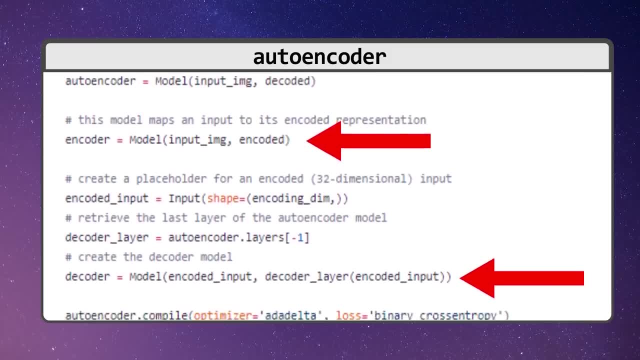 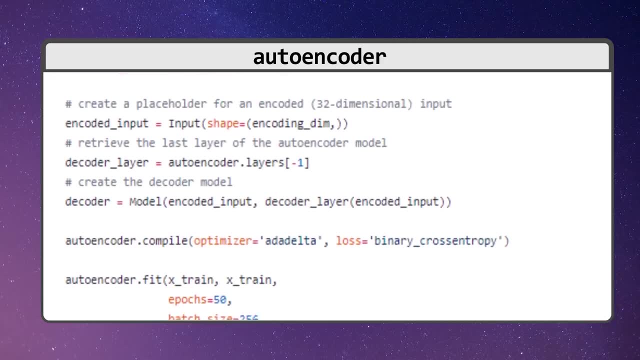 and as the decoder. And this model is just a simple neural network. we're only calling it an autoencoder because we're feed it the inputs- input data as the labels. since we don't have any labels, The reconstructed results will look very similar to the original input data after we're done. 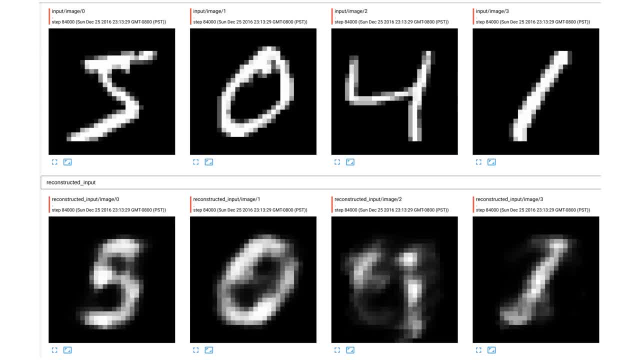 training. Sometimes, though, the model could overfit on the input data, and, in order for it to be able to learn a better, more robust representation to the input data, we can manually add some noise, And this is called a denoising autoencoder. 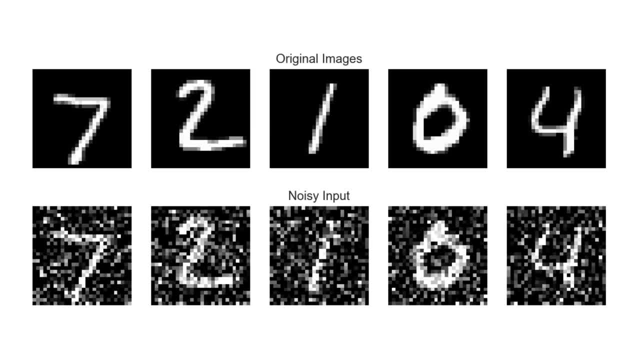 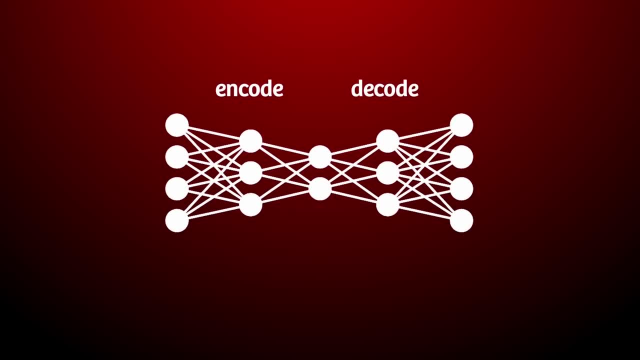 The amount of noise to apply to the input usually takes the form of a percentage. There are so many different types of autoencoders we could make, but one in particular that I really like is called the variational autoencoder. This learns a latent variable model of its input data. 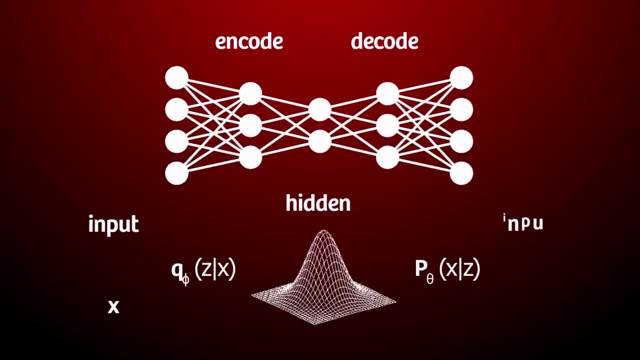 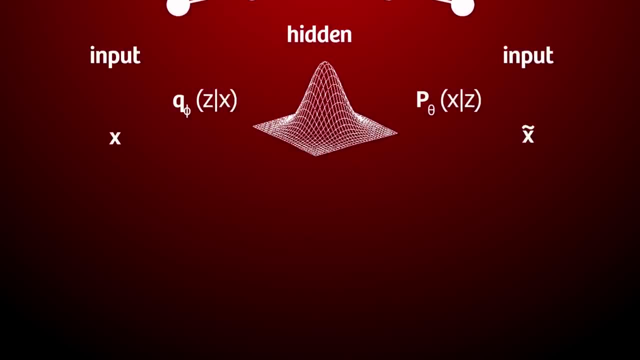 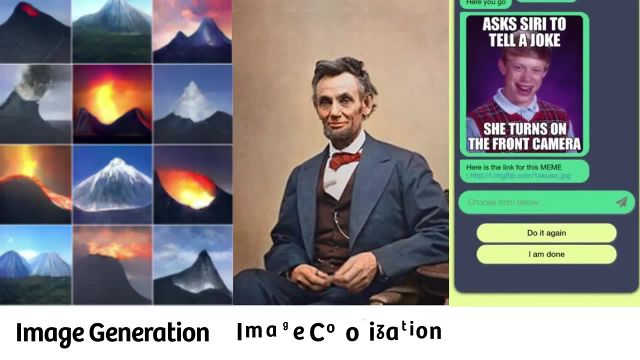 Instead of letting the network learn some function, we're learning the parameters of a probability distribution that models our data. Then we can sample points from this distribution and generate new input data samples, meaning a VAE can be considered a generative model. This lets us create all sorts of new images and videos that have never existed before. 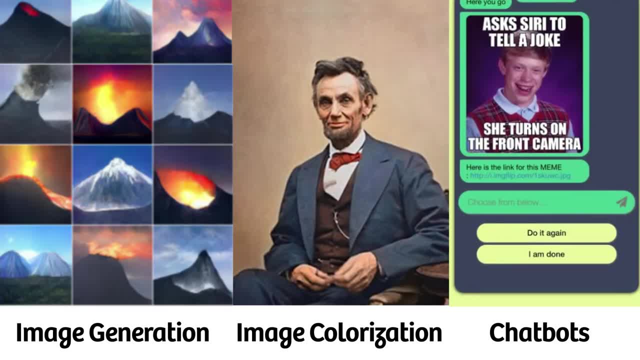 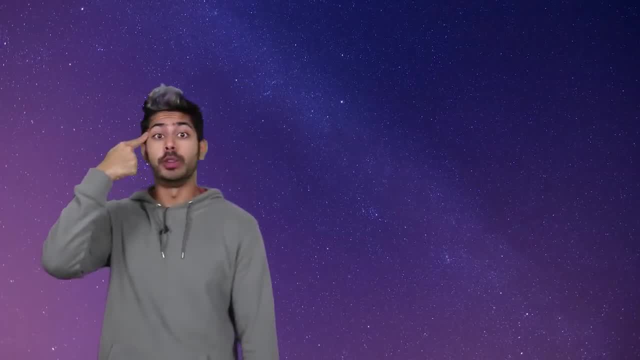 Image colorization chatbots- VAEs- are right up there with generative adversarial networks. as one of my top five favorite deep learning models, Three points to encode in your biological neural network from this video. Neural networks can slowly approximate any function that maps inputs to outputs through. 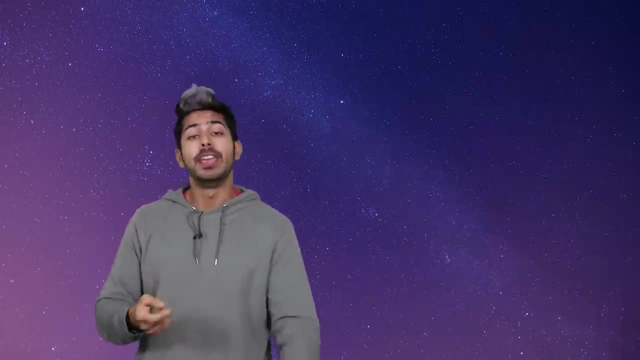 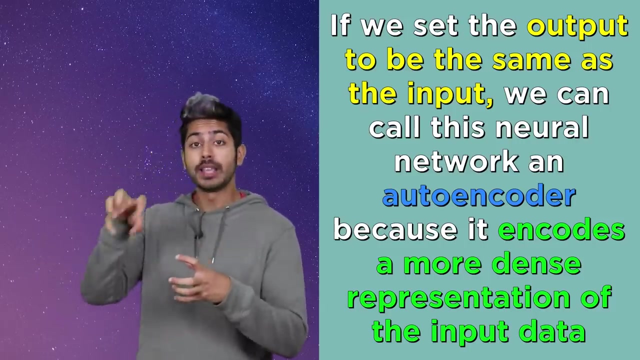 an iterative optimization process, also called training. If we set the output to be the same as the input, we can call this neural network an autoencoder, because it encodes a more dense representation of the input data. That's it, And there are many types of autoencoders we could make.